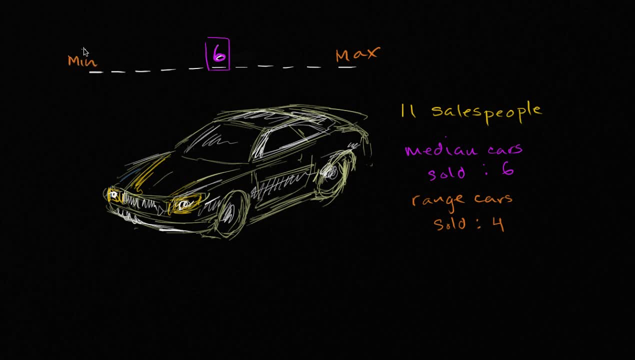 because we've sorted them all out and this is our min right over here. our range is going to be our max minus minus our min. So let me write that down. So you take your min and your max, you have your range. 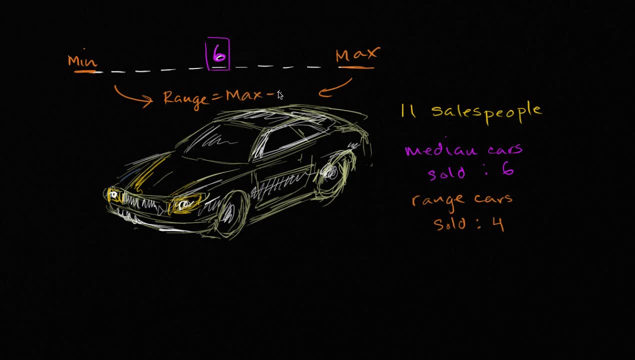 range is equal to the maximum minus the minimum, And they're telling us that that is four. this range is four, So the maximum minus the minimum, the difference between the number of cars that the most productive salesperson sold and the number of cars that the least productive. 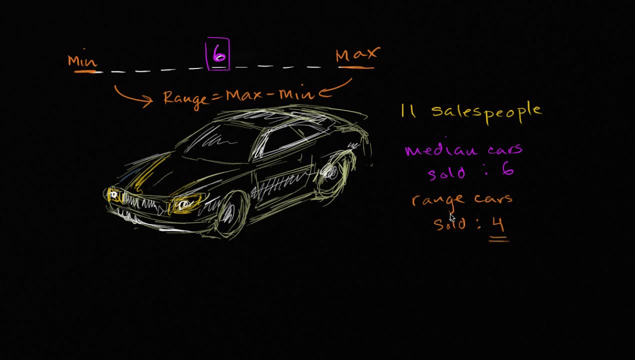 salesperson sold, that difference is going to be four. So, given all of those assumptions, given all of that information, I'm now going to give you a statement. And our challenge is: if we assume everything I just said is true, is this statement going to be true? 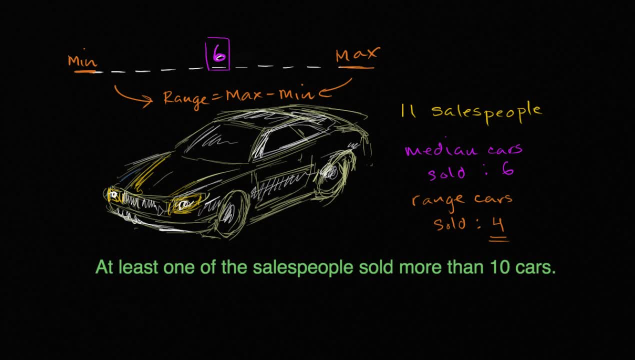 Or is this statement going to be false Or do we not know? So let me write this down. So is this going to be true, false, false or do we not know? Do we not have enough information to say it's for sure going to be true? 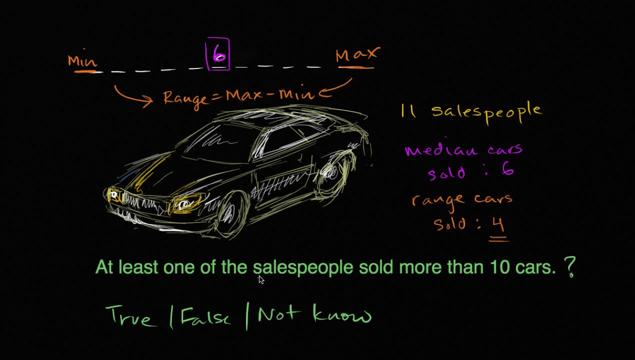 for sure going to be false, or for sure, we don't know- And so I encourage you to pause the video now and try it out. All right, so let's work through it together. This is kind of a fun puzzle here, where we've been given some clues. 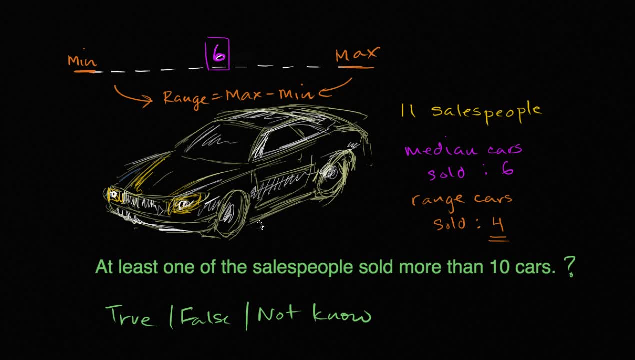 and then we have a statement and we figure: can we make the statement? Can we say it's true, Or can we say for sure that it's false, Or do we just not know? So a couple of ways to tackle it. One way to tackle it is: well look. 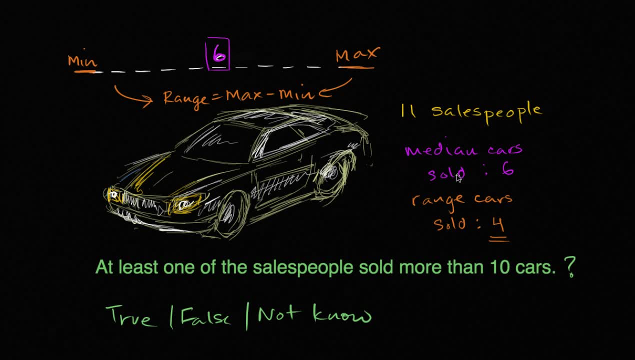 one of the salespeople must have sold six cars. If the median sold is six and there's 11 salespeople here- the middle number here if we order it- one of them must have sold six cars If we had an even number here. 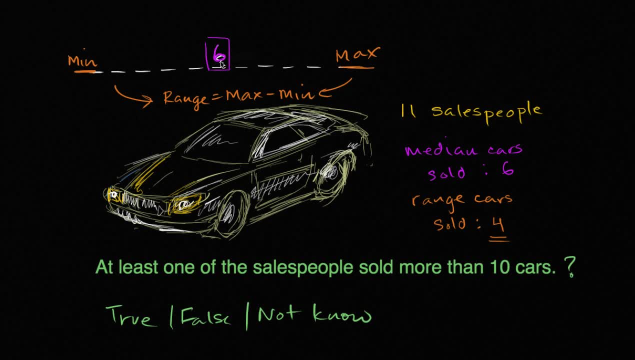 then that would be the average of the two middles. but if we have an odd number here, that is literally the middle number of cars that somebody- the middle number of cars- sold. So someone sold six cars. So if we assume, if we assume, 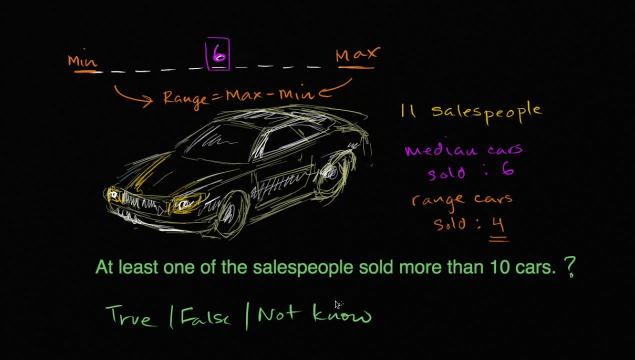 we're trying to find a world where someone sold more than 10 cars. So if someone sold six cars, is there a way, with a range of four, that someone sold more than 10?? Well, let's just think about it. Let's just assume that the min is six. 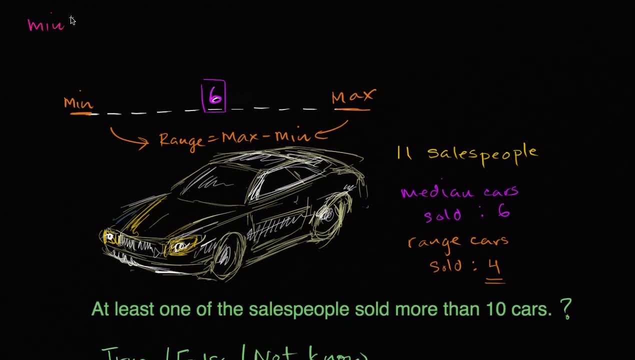 We don't know that the min is six, but let's just try it out. If the minimum is six, if the minimum is six, what's the maximum going to be? Well, remember the range the range is equal to. we know that the range is four. 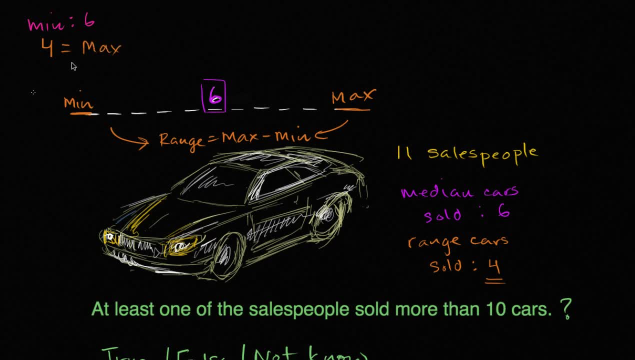 the range is equal to the maximum minus the minimum, Maximum minus the minimum, And so the maximum in this case would be 10, would be 10.. Max would be equal to: would be equal to 10.. If the min is equal to six, 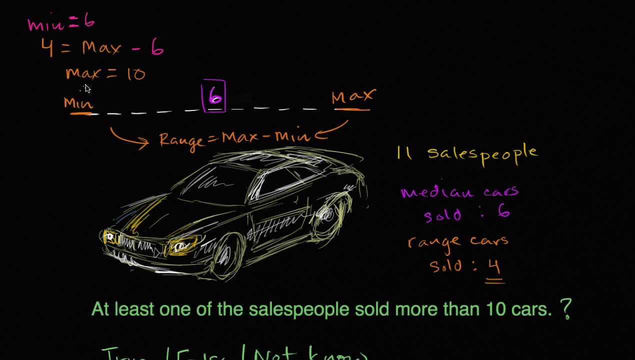 and instead of colons I'm gonna write an equal sign. If the min is equal to six, then the max at most can be equal to 10.. And we can't take a higher min because we know that the six six is going to be one of the values. 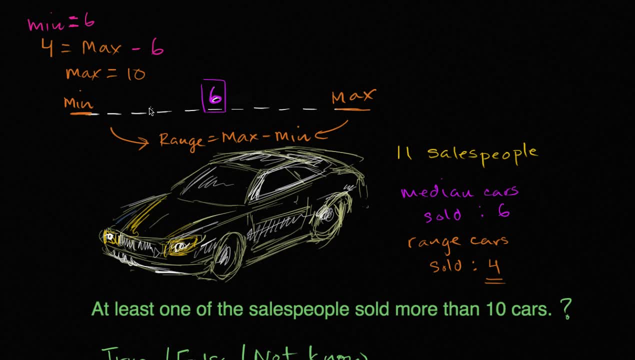 We could try a lower minimum value. We could say the minimum value is five or four, or three, or two or one, but then the maximum would go down even more Because, remember, the maximum is no more than four larger than the minimum. 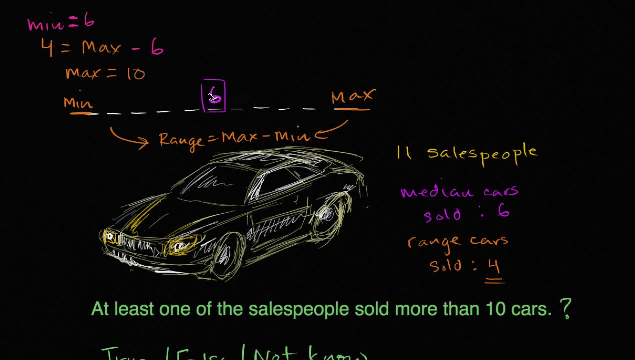 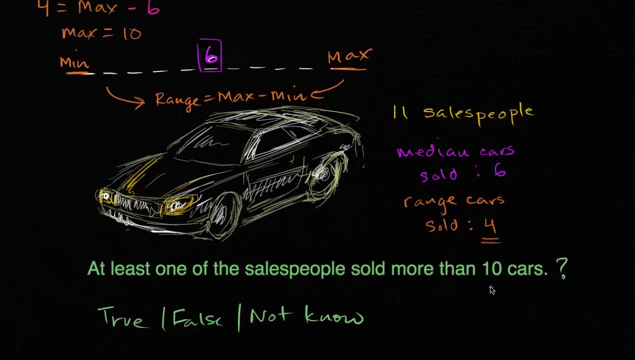 So if we assume six and we know that one of the salespeople sold six cars, then the maximum that any of the salespeople could have sold is 10.. And so the statement: at least one of the salespeople sold more than 10 cars. 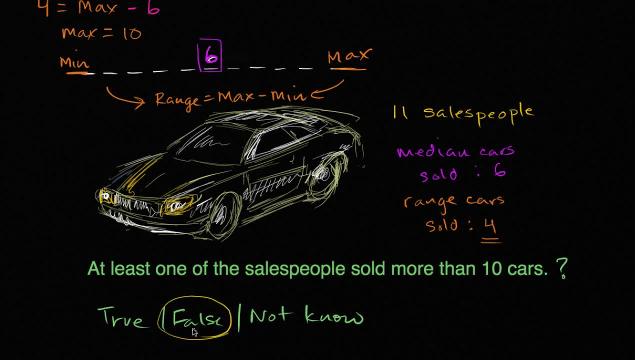 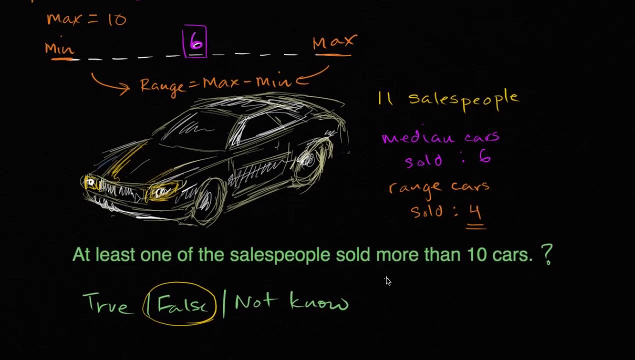 that's gotta be false. That's gotta be false. Now there's another way that you could think about it. You could assume that someone sold more than 10.. You could assume in the last example or the last way of thinking about it. 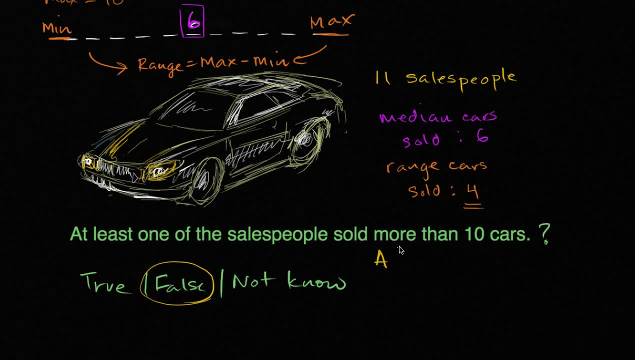 we assumed that the min was six. but now let's just assume. let's just assume that someone sold. let's just try it out, Let's see if it's possible. Let's just assume that the max is 11, that someone sold more than 10 cars. 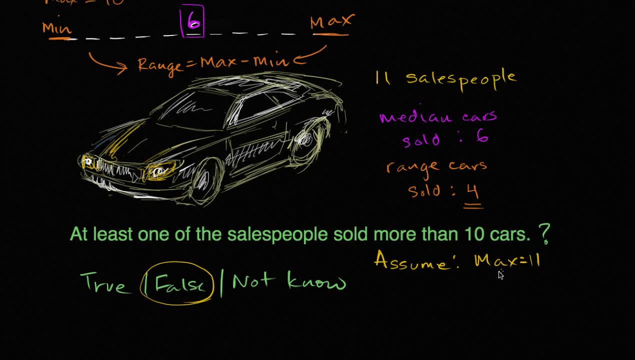 If the max is equal to 11, what's the min going to need to be? Well, we just have to remind ourselves: range is equal to max minus min. So four is equal to the maximum: 11 minus min, Minus the minimum.